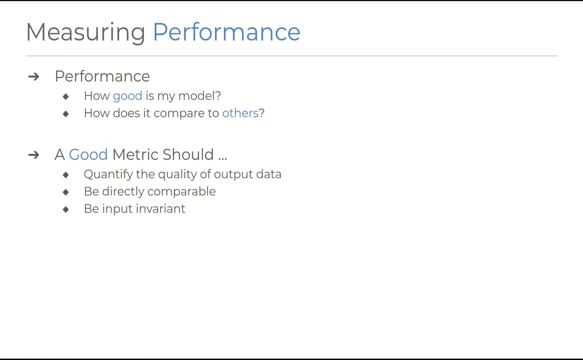 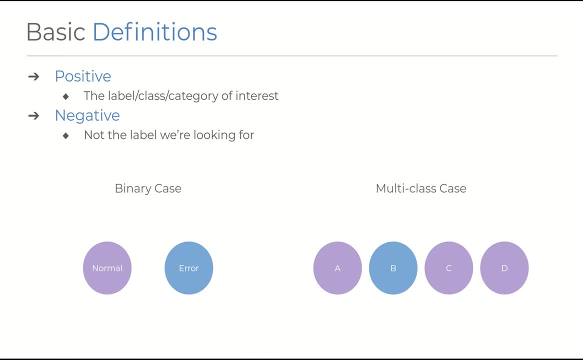 shouldn't have a biased advantage over any other That sort of problem. But before we can get started with the metrics we have to go over some very basic definitions of the categories that we can go group the output into. So say we have a system that makes a prediction about the class of an object. 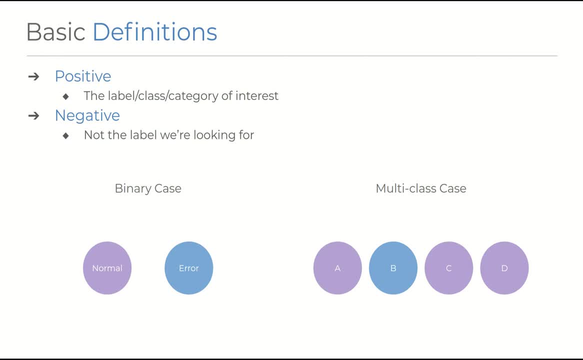 We say that a positive case is when the label or category is the one we're interested in. For example, say that we're looking at detecting errors in a dataset. If we're interested in metrics measuring the performance of identifying the error case. 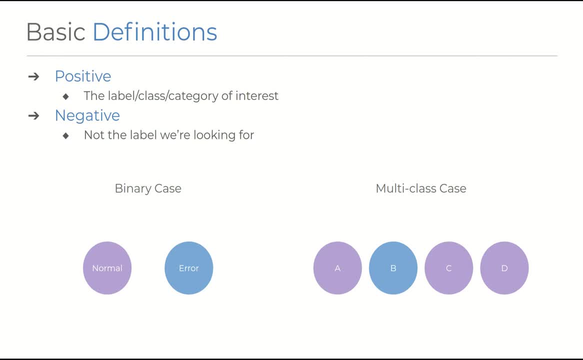 we would class that as the positive case and normal operation as negative, which is straightforward. Another example is classifying items into four different categories of A, B, C and D, And we want to measure the performance with regards to the class of, say, B. 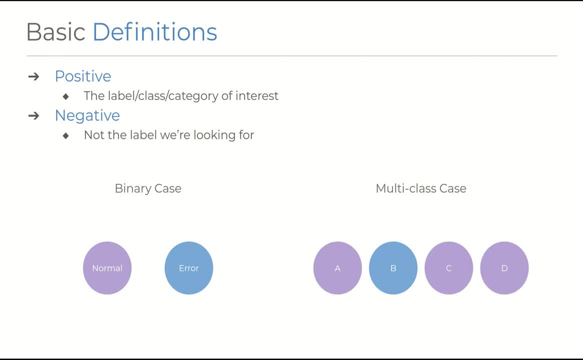 Then, in this case, B is the positive one here and anything else- A, C and D- are negative cases. Again, extremely straightforward. But the key point here is that all of our metrics are specific to the class we choose to define as being positive. 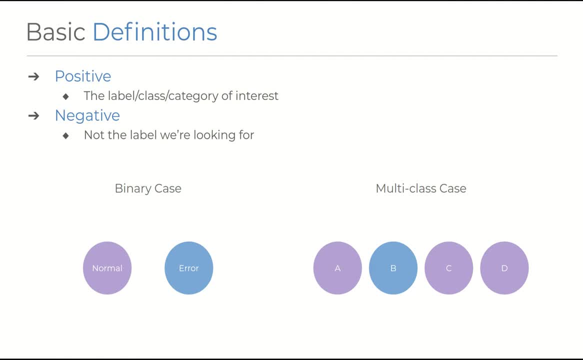 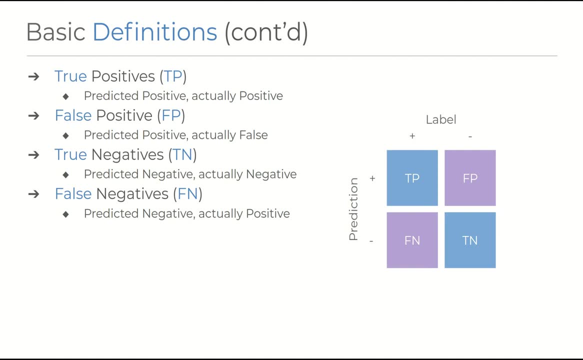 This distinction becomes important and apparent as we explore the different metrics, especially for the multi-class systems. So, based on this, we can further divide the predictions we make on some data into four useful groups. When a label is positive and we predict it to be positive. 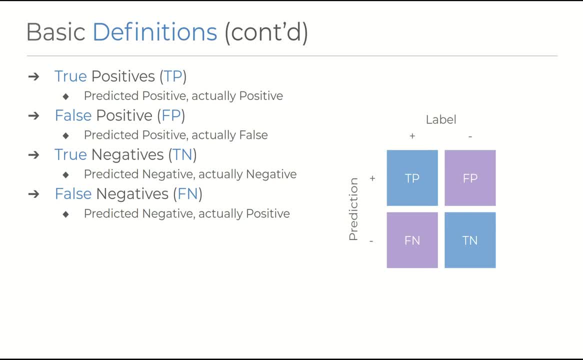 we call that a true positive case. And, conversely, if our positive predictions label was actually negative, then that is a false positive, And so on. it goes for true negatives and false negatives. These values are usually expressed as the actual number of predictions that fall into each category. 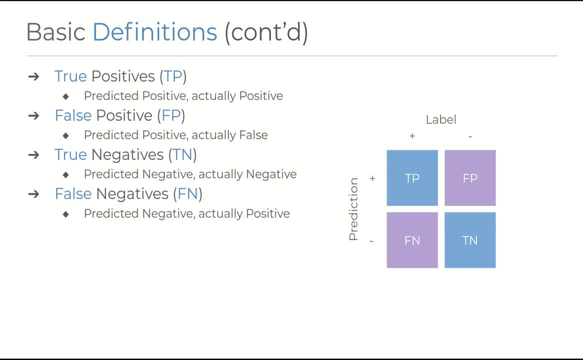 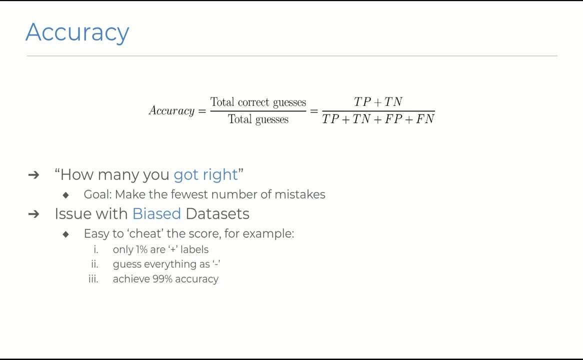 or as a percentage with regards to all of the predictions that were made. So we'll begin with the most basic metric and formally define what accuracy is. Almost everyone should have a near-instinctual understanding of what this is, but let's go through it step by step anyway. 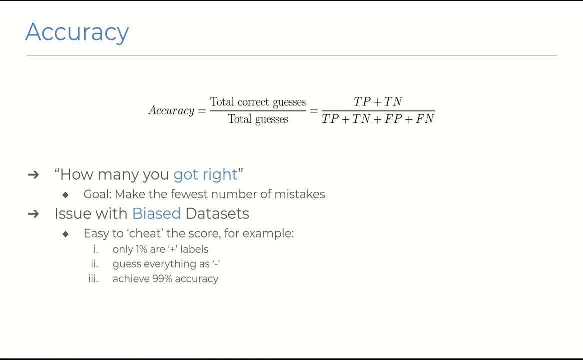 So all we have to do to measure the accuracy of our system is to count the number of right answers and express it as a portion of all the answers we gave. More formally by our previous definitions, the accuracy of our system is given by the number of true positives and true negatives over the entire prediction set. 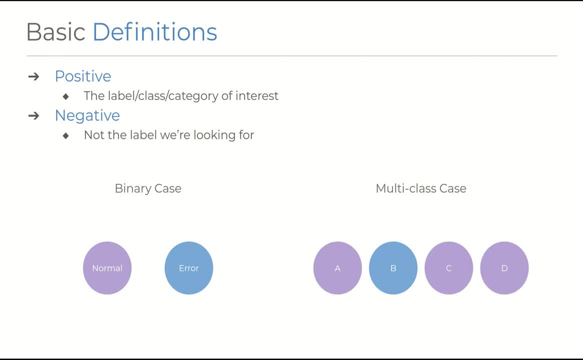 Then, in this case, B is the positive one here and anything else- A, C and D- are negative cases. Again, extremely straightforward. But the key point here is that all of our metrics are specific to the class we choose to define as being positive. 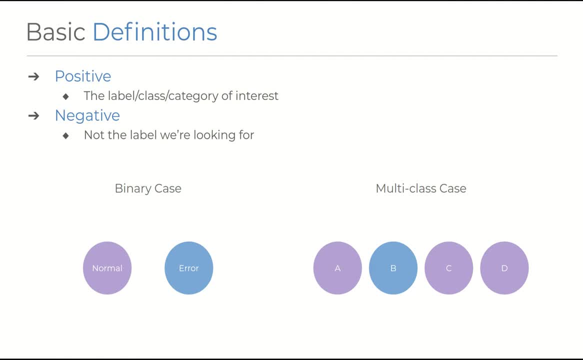 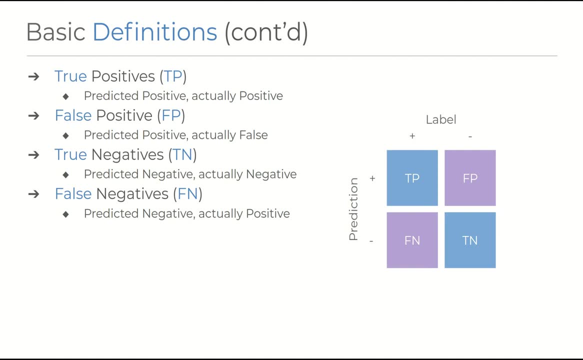 This distinction becomes important and apparent as we explore the different metrics, especially for the multi-class systems. So, based on this, we can further divide the predictions we make on some data into four useful groups. When a label is positive and we predict it to be positive. 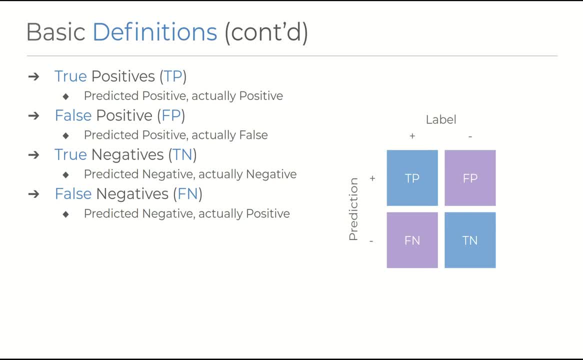 we call that a true positive case. And, conversely, if our positive predictions label was actually negative, then that is a false positive, And so on. it goes for true negatives and false negatives. These values are usually expressed as the actual number of predictions that fall into each category. 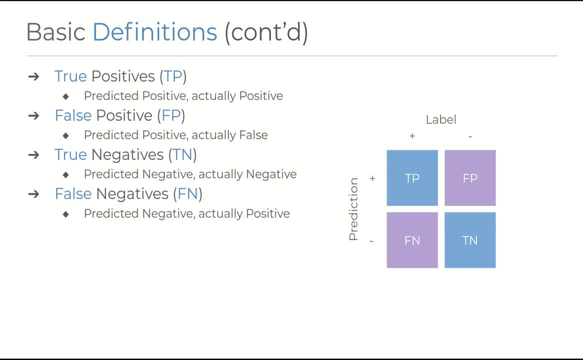 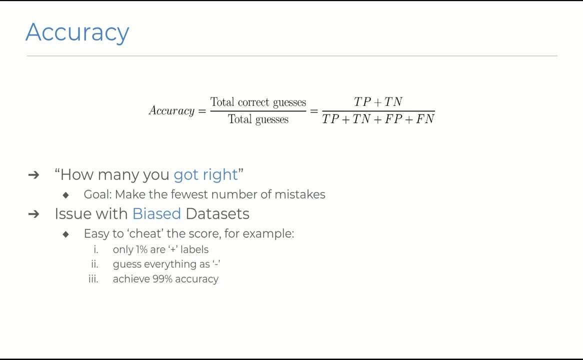 or as a percentage with regards to all of the predictions that were made. So we'll begin with the most basic metric and formally define what accuracy is. Almost everyone should have a near-instinctual understanding of what this is, but let's go through it step by step anyway. 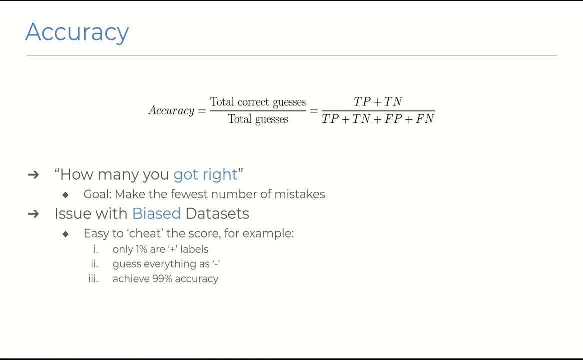 So all we have to do to measure the accuracy of our system is to count the number of right answers and express it as a portion of all the answers we gave. More formally by our previous definitions, the accuracy of our system is given by the number of true positives and true negatives over the entire prediction set. 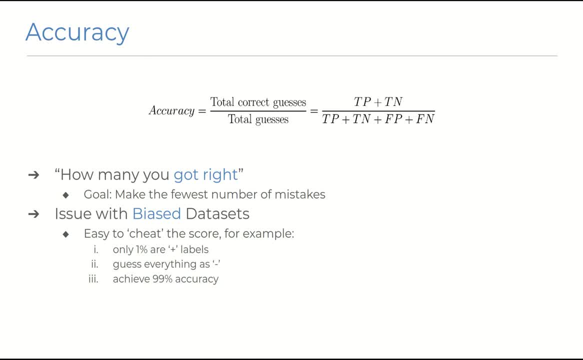 Accuracy essentially tells us how many answers we got right out of all the guesses we've made and notably, this is without any regard for whether the guesses were about positive or negative labels. But of course, there's a glaring issue with this straight-up accuracy in measuring performance. 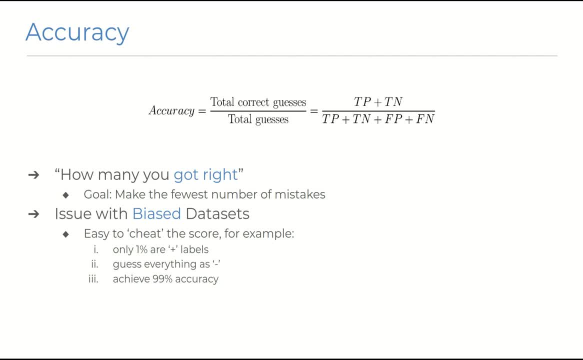 and that becomes apparent when we're dealing with biased datasets. So imagine we have a dataset that's characterized by almost all of the labels being negative labels and only say 1% of them are actually positive. If the model then decides to only output negative predictions and absolutely zero positive guesses, 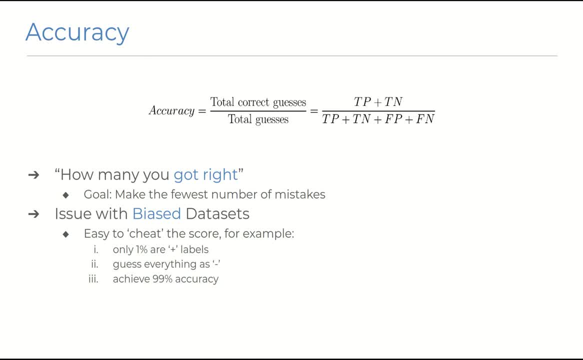 Accuracy essentially tells us how many answers we got right out of all the guesses we've made and notably, this is without any regard for whether the guesses were about positive or negative labels. But of course, there's a glaring issue with this straight-up accuracy in measuring performance. 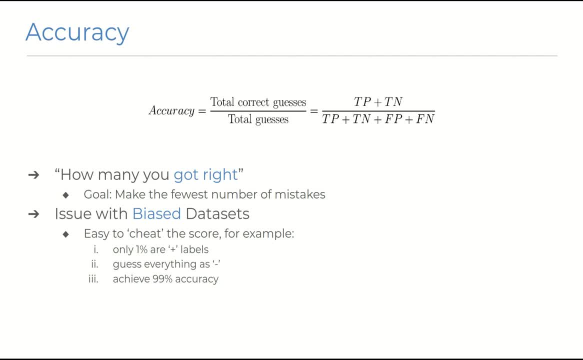 and that becomes apparent when we're dealing with biased datasets. So imagine we have a dataset that's characterized by almost all of the labels being negative labels and only say 1% of them are actually positive. If the model then decides to only output negative predictions and absolutely zero positive guesses, 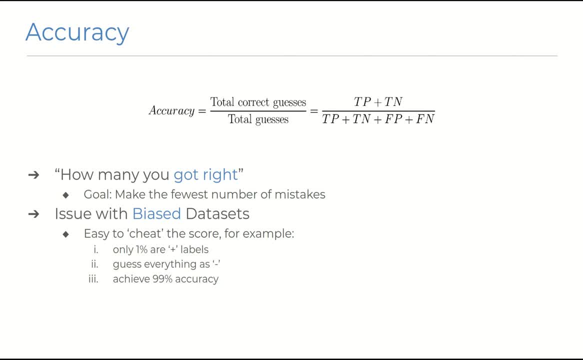 it will still be counted as having a 99% accuracy score. And this isn't just a toy example. when you think of, say, disease testing or predicting system faults, The normal case in these scenarios will usually vastly outnumber any abnormal examples. But even datasets with, you know, milder biases can have their performance metrics skewed. 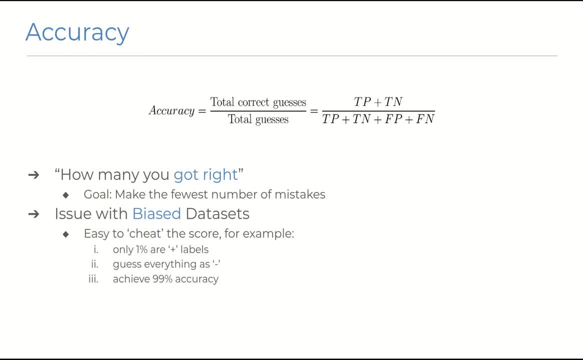 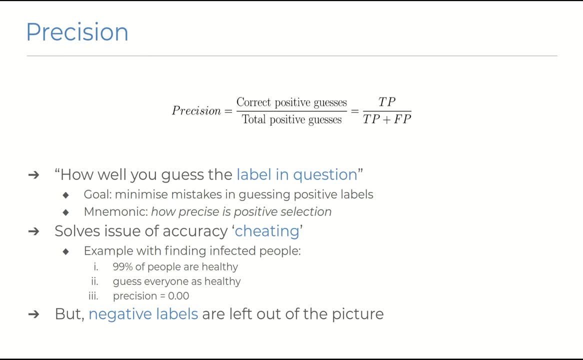 in this manner, just a little more subtly, And this is where a metric like precision comes into play. We can say that precision is a measure of how well you've guessed the label that we're interested in, namely the positive case, And we calculate it by dividing the number of correct positive guesses by all the positive guesses we've made. 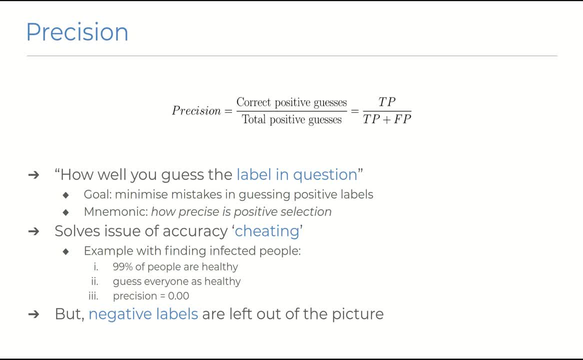 Formally the true positive count over the true positive plus false positive count. The goal of a system that optimizes for this metric would be to make as few mistakes as possible when guessing the positive labels And looking back at the example where a system would just guess negative for everything. 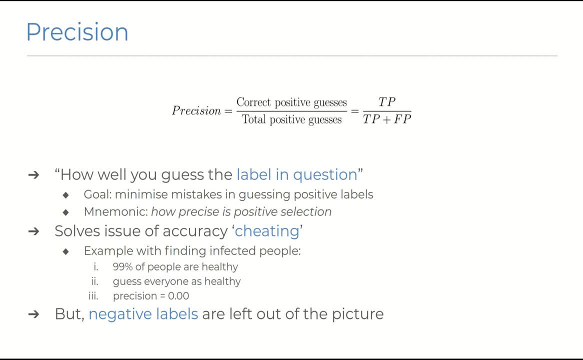 we'll see that the precision score penalizes the model with the score of zero because it has failed to guess any positive labels whatsoever. However, precision still doesn't paint the entire picture because it doesn't take into account any of the negative labels. 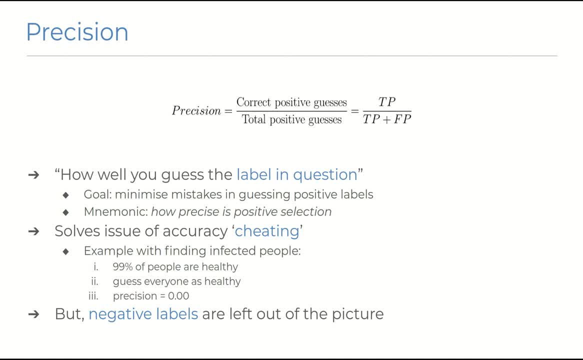 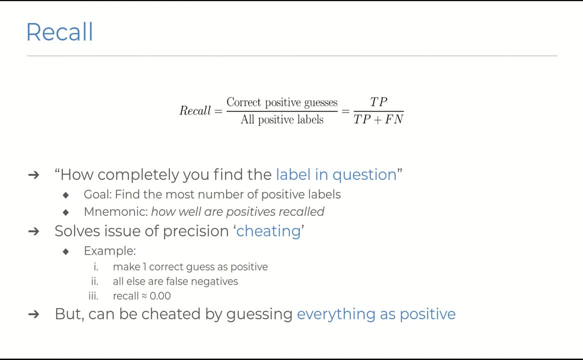 And further. this metric can also be defeated if the system just makes one correct positive guess and doesn't make any more predictions, giving it a 100% score. So now we have recall, And this is like a counterpart to precision, and it's notably different in that it takes the negative labels into the equation. 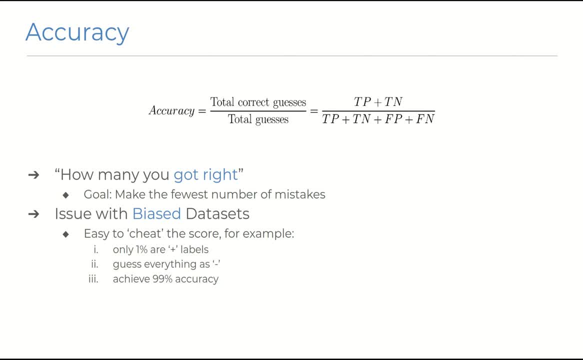 it will still be counted as having a 99% accuracy score. And this isn't just a toy example. when you think of, say, disease testing or predicting system faults, The normal case in these scenarios will usually vastly outnumber any abnormal examples. But even datasets with, you know, milder biases can have their performance metrics skewed. 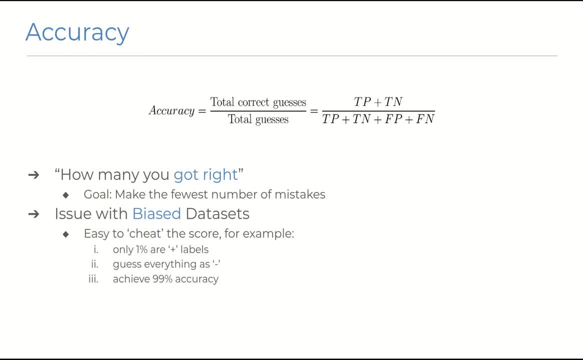 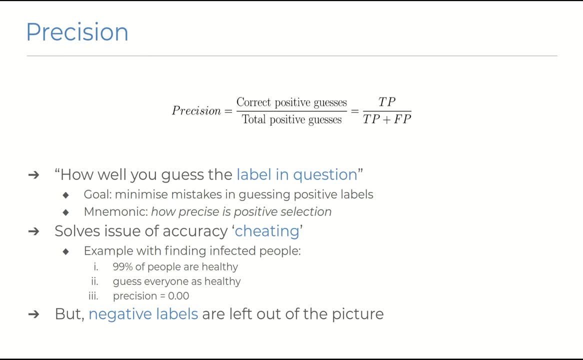 in this manner, just a little more subtly, And this is where a metric like precision comes into play. We can say that precision is a measure of how well you've guessed the label that we're interested in, namely the positive case, And we calculate it by dividing the number of correct positive guesses by all the positive guesses we've made. 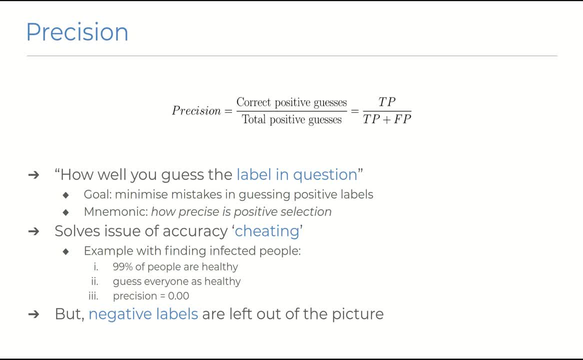 Formally the true positive count over the true positive plus false positive count. The goal of a system that optimizes for this metric would be to make as few mistakes as possible when guessing the positive labels And looking back at the example where a system would just guess negative for everything. 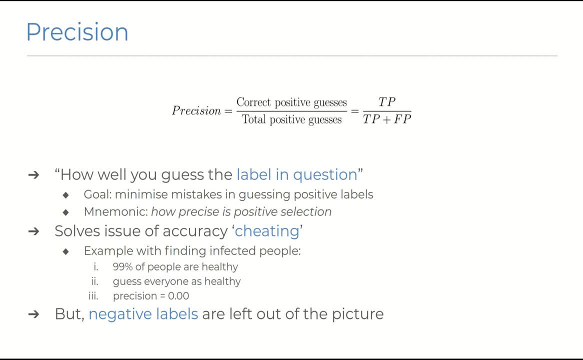 we'll see that the precision score penalizes the model with the score of zero because it has failed to guess any positive labels whatsoever. However, precision still doesn't paint the entire picture because it doesn't take into account any of the negative labels. 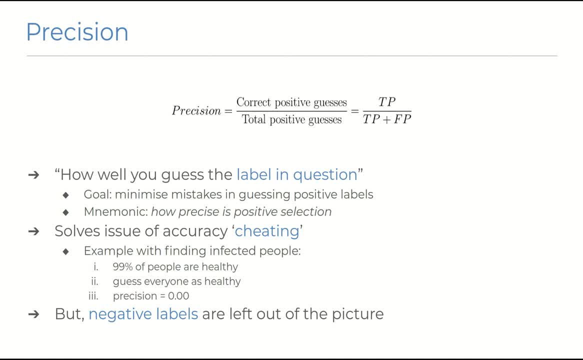 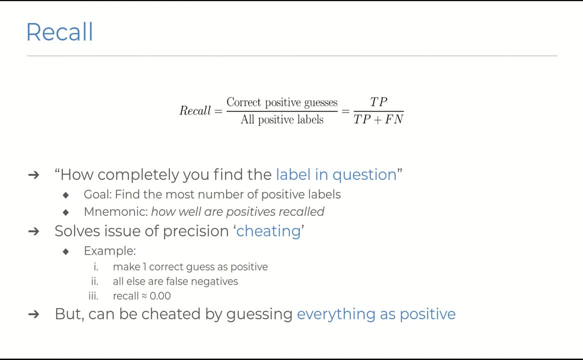 And further. this metric can also be defeated if the system just makes one correct positive guess and doesn't make any more predictions, giving it a 100% score. So now we have recall, And this is like a counterpart to precision, and it's notably different in that it takes the negative labels into the equation. 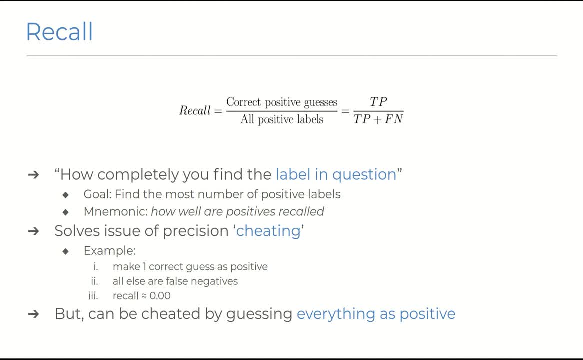 It asks the question of how many positive labels you've found out of the total number of positive labels that exist, almost directly countering the issue seen with precision, And, of course, the equation for this comes down to the number of correctly predicted positive labels. 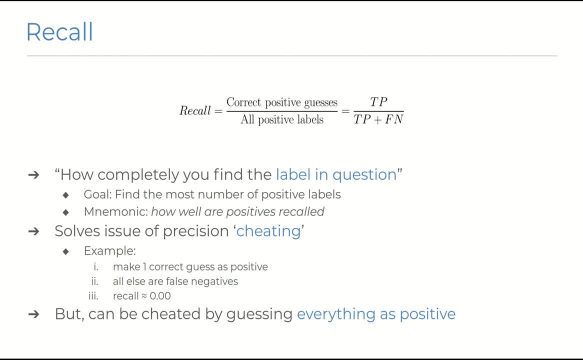 divided by the number of positives you've got correct plus the number of positives you got wrong. The goal of the system then becomes to try and find every positive label there is to be found. But, alas, recall still has a problem, And this is skewing the score by being liberal with labeling anything as positive. 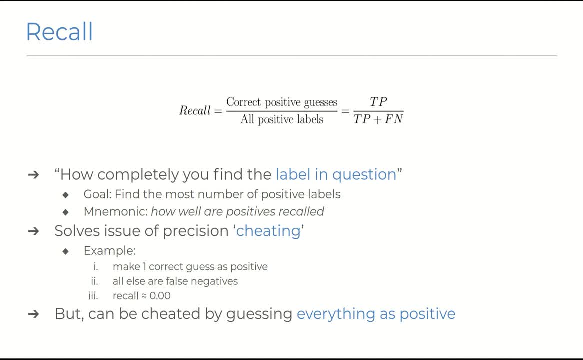 It asks the question of how many positive labels you've found out of the total number of positive labels that exist, almost directly countering the issue seen with precision, And, of course, the equation for this comes down to the number of correctly predicted positive labels. 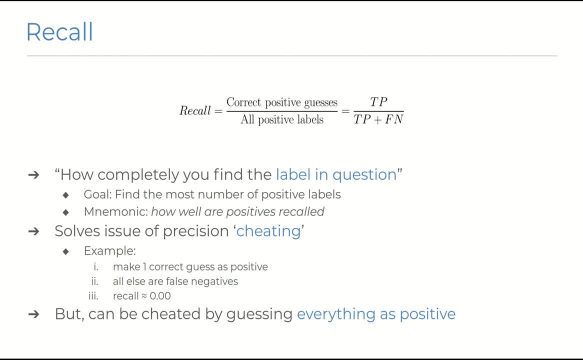 divided by the number of positives you've got correct plus the number of positives you got wrong. The goal of the system then becomes to try and find every positive label there is to be found. But, alas, recall still has a problem, And this is skewing the score by being liberal with labeling anything as positive. 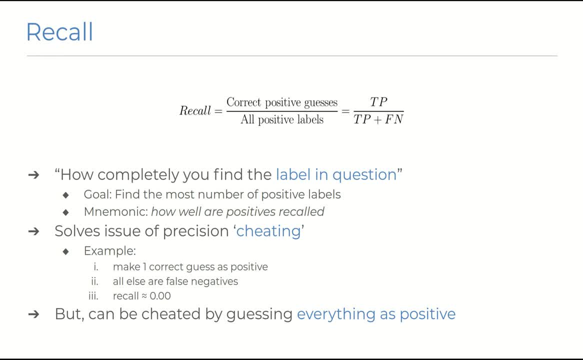 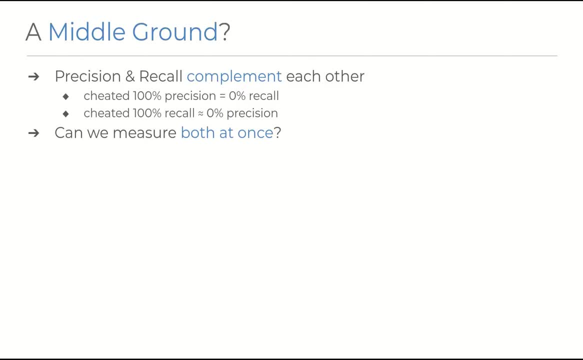 So, in the extreme case of this, simply labeling everything as positive will result in no false negatives and thus a perfect recall score. It should be clear by now that the metrics of precision and recall alone have some very severe shortcomings, but also the fact that one sort of prevents cheating of the other score. 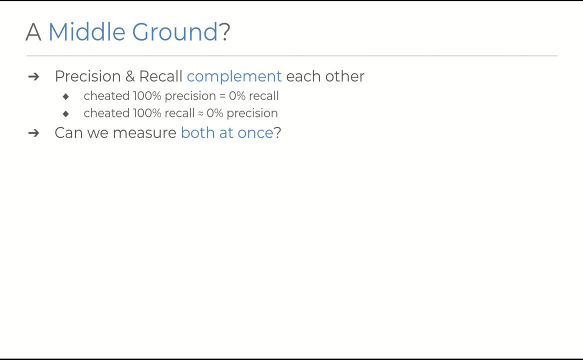 Cheating to get a recall of 100% will result in a precision of 0, and vice versa. In this way, these two metrics sort of complement each other. So the question arises then, if we can design a system so that it optimizes for both of these scores at the same time. 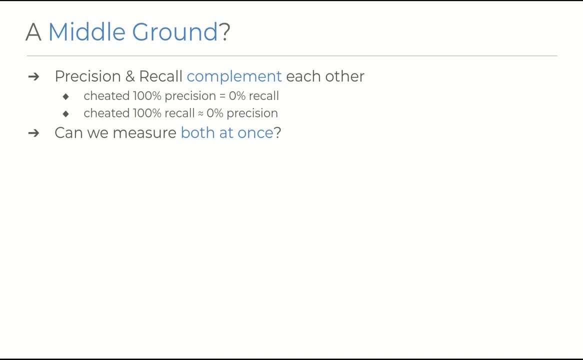 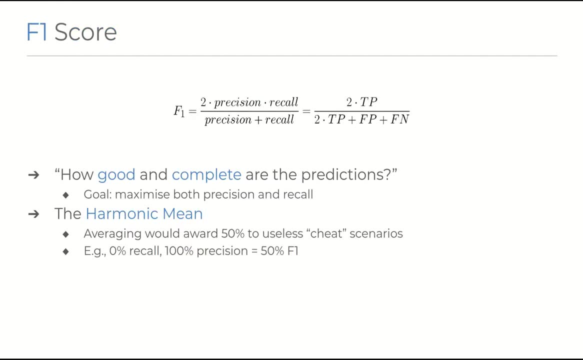 Namely, we want to make something that incorporates both the quality of the predictions and the completeness of the predictions into a single score, And this is where the F1 score comes in. The F1 score is defined to be the harmonic mean between precision and recall. 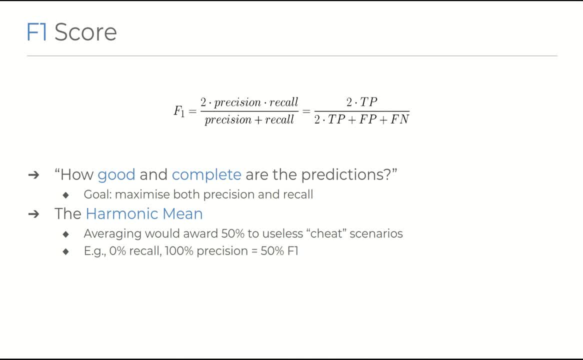 and the score essentially asks, as said earlier, how good the quality of the predictions are and how completely we have predicted the labels from the dataset. Very importantly, the F1 score doesn't simply use an arithmetic average to combine the score, In fact. 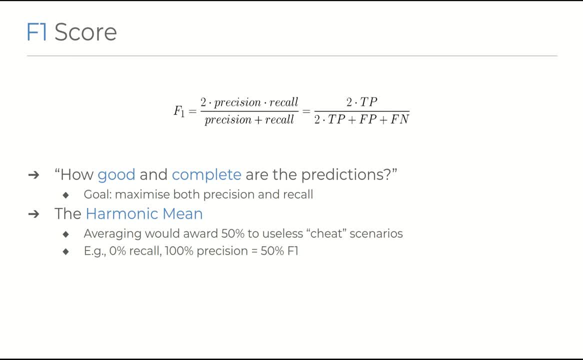 this would be pretty detrimental in the so-called cheating cases we discussed earlier, where a model that just predicts negative for everything still gets awarded a 50% score. by average, The harmonic mean weights the score towards the lower of the two components, and this essentially penalizes precision and recall. 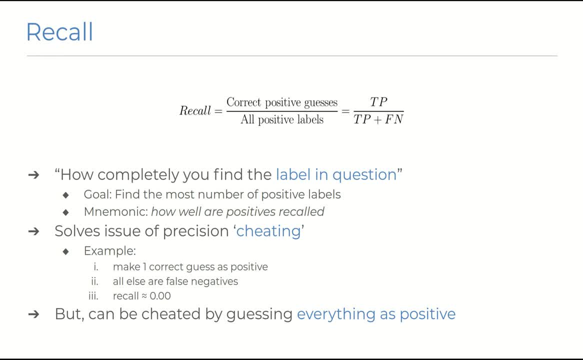 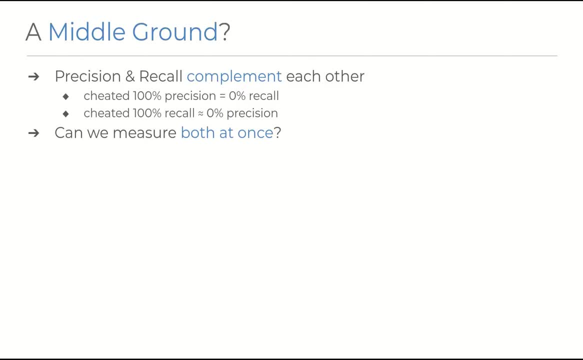 So, in the extreme case of this, simply labeling everything as positive will result in no false negatives and thus a perfect recall score. It should be clear by now that the metrics of precision and recall alone have some very severe shortcomings, but also the fact that one sort of prevents cheating of the other score. 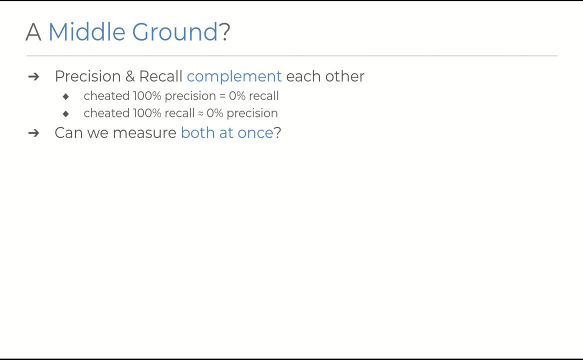 Cheating to get a recall of 100% will result in a precision of 0, and vice versa. In this way, these two metrics sort of complement each other. So the question arises then, if we can design a system so that it optimizes for both of these scores at the same time. 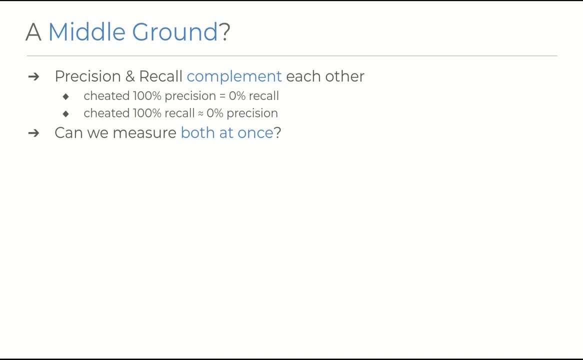 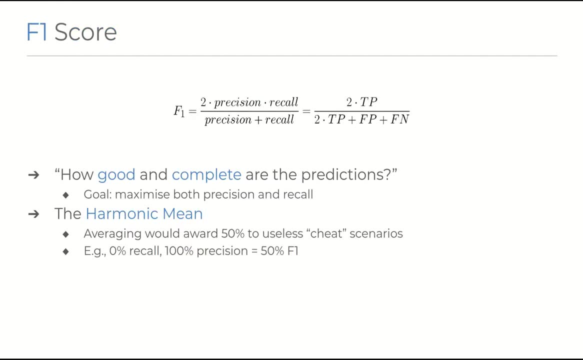 Namely, we want to make something that incorporates both the quality of the predictions and the completeness of the predictions into a single score, And this is where the F1 score comes in. The F1 score is defined to be the harmonic mean between precision and recall. 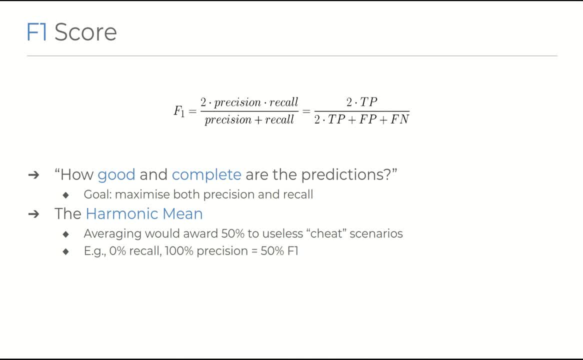 and the score essentially asks, as said earlier, how good the quality of the predictions are and how completely we have predicted the labels from the dataset. Very importantly, the F1 score doesn't simply use an arithmetic average to combine the score, In fact. 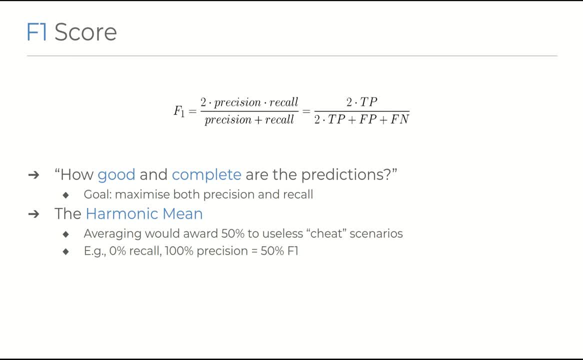 this would be pretty detrimental in the so-called cheating cases we discussed earlier, where a model that just predicts negative for everything still gets awarded a 50% score. by average, The harmonic mean weights the score towards the lower of the two components, and this essentially penalizes precision and recall. 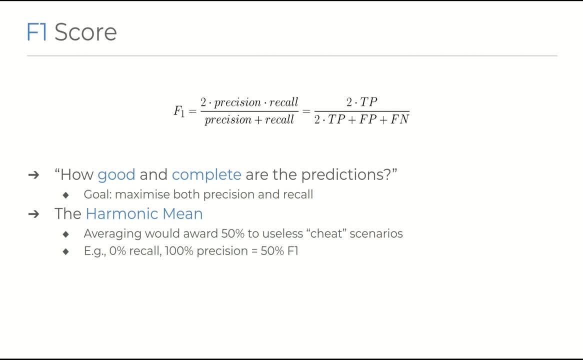 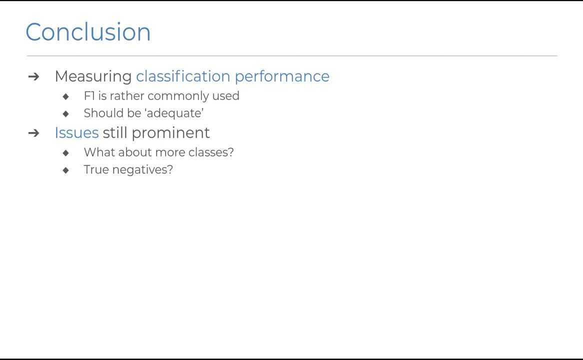 disagreeing with each other too much and correctly reflects when either of them falls too close to the value of zero. And that's basically it. The F1 score is definitely one of the most common metrics by which we compare our systems and, for most cases, will serve as a good indicator of how healthy your model is performing. 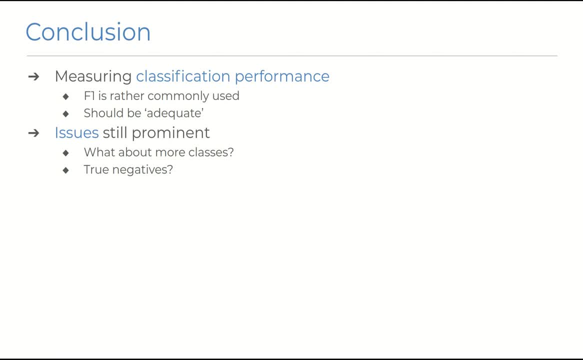 However, there are still some cases where it won't be so adequate, especially when we have to deal with multi-class systems, for which the performance with regards to each different class is equally important. And, by extension, this metric doesn't have true negatives in its calculation.